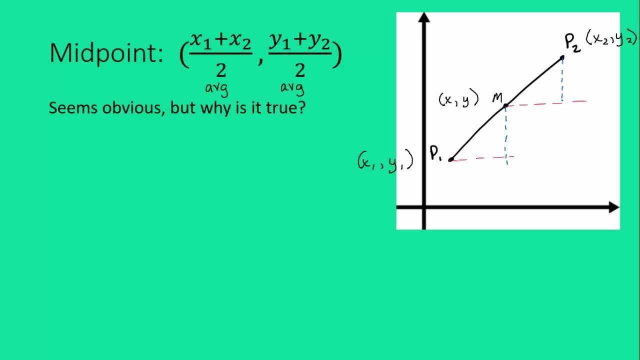 in the picture, There's some horizontal lines and there's some mostly vertical lines. Okay, what do we know about these two right triangles? The red lines are parallel and the blue lines are parallel right, Keep that in mind. Since the red lines are parallel, P1- P2 is a transversal that crosses them. 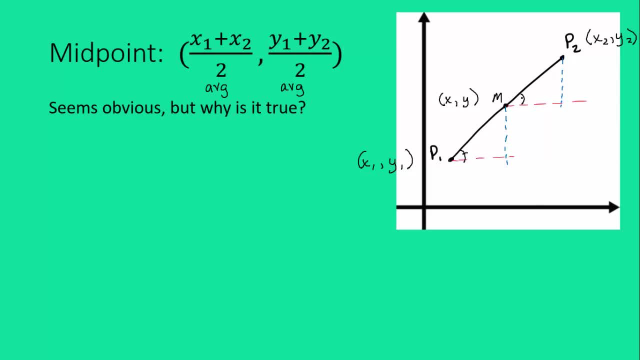 both, so we can say that these two angles are congruent. Similarly, the vertical lines are also parallel and P1- P2 is a transversal across them as well, so we know that these angles are also congruent. Well, we were given the information in the first place that M is equidistant between P1 and P2.. 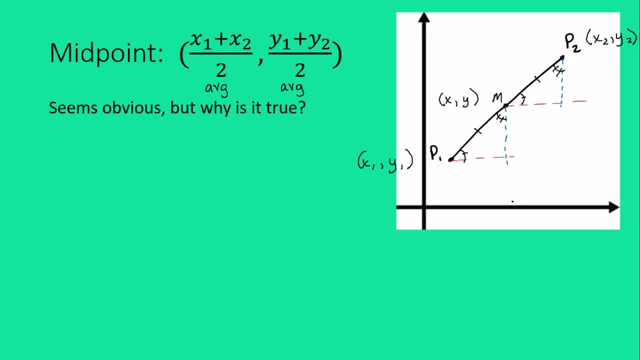 So we also know that these are congruent, and so now we have angle side angle. Let's label these new points also so that we can name those triangles. So the triangles are P1, MA and MP2 B, and those are congruent and so all their parts are. 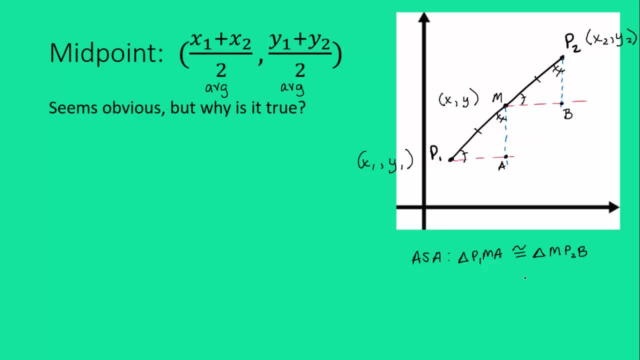 congruent that correspond. That's going to help us in our proof. So now what I'm going to do is I'm going to use the other parts of the triangles to make some equations using the coordinates and then figure out if we can prove this. 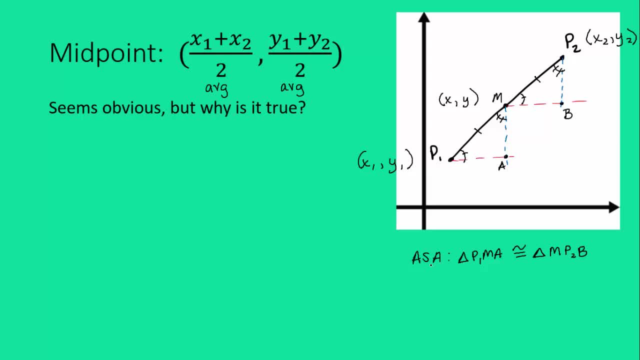 midpoint formula. So the first thing I'm going to do is look at those two red lines. Not only are they parallel, but now, because they're parts of two congruent triangles, we know that they are congruent as well. The distance from P1. 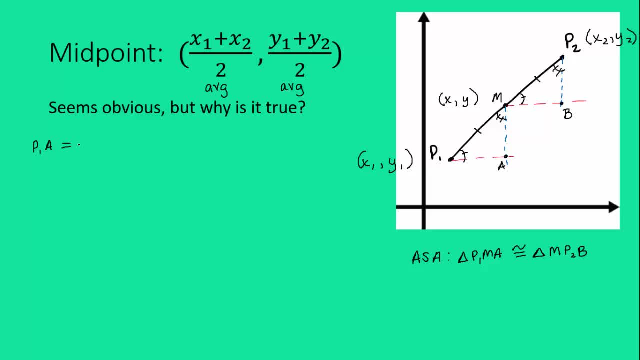 to A is equal to the distance from M to B. We can also say that those blue line segments are congruent, so the distance from M to A is equal to the distance from P2 to B. Alright, using using those equations, we're going to make equations using our coordinates. Well, we need to. 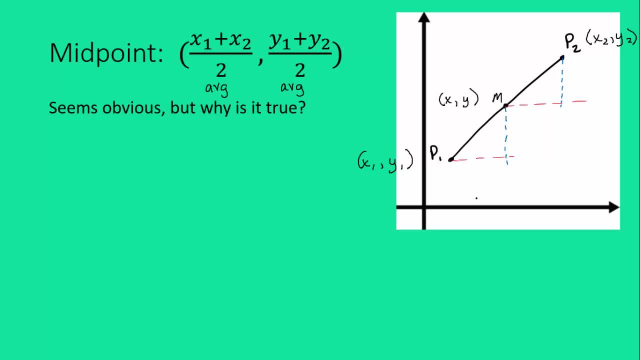 The red lines are parallel and the blue lines are parallel, right, Keep that in mind. Since the red lines are parallel, P1, P2 is a transversal that crosses them both, so we can say that these two angles are congruent. 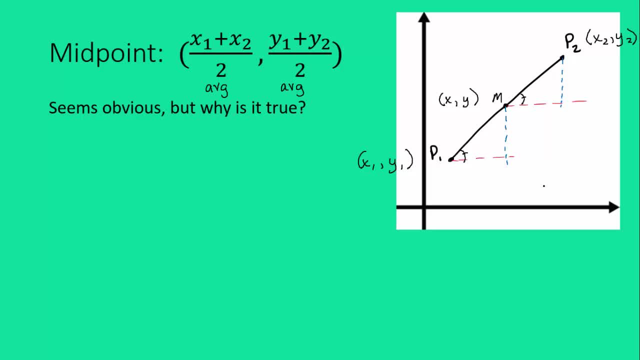 Similarly, the vertical lines are also parallel and P1, P2 is a transversal across them as well, so we know that these angles are also congruent. Well, we were given the information in the first place that M is equidistant between P1 and P2,. 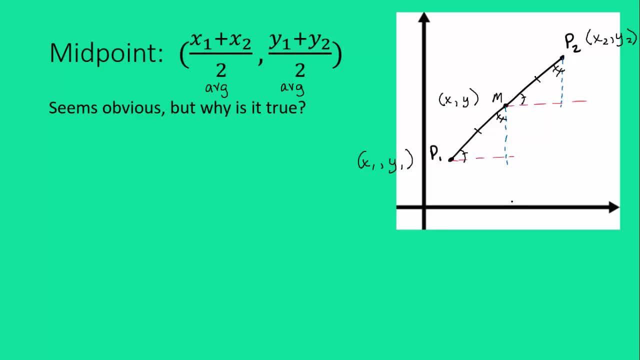 so we also know that these are congruent. And so now we have angle-side-angle, Let's label these new points also so that we can name those triangles. So the triangles are P1MA and MP2B and those are congruent, and so all their parts are congruent. that correspond. 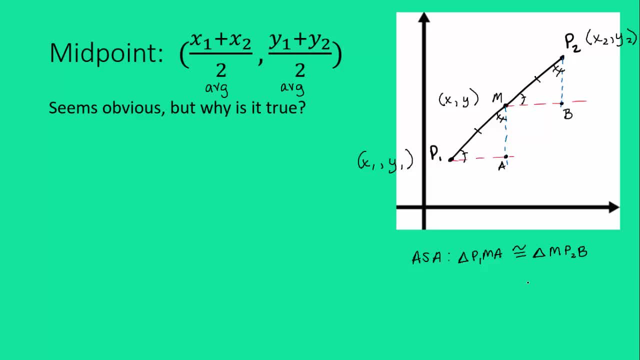 That's going to help us in our proof. So now, what I'm going to do is I'm going to use the other parts of the triangle. So what I'm going to do is I'm going to use the other parts of the triangle. 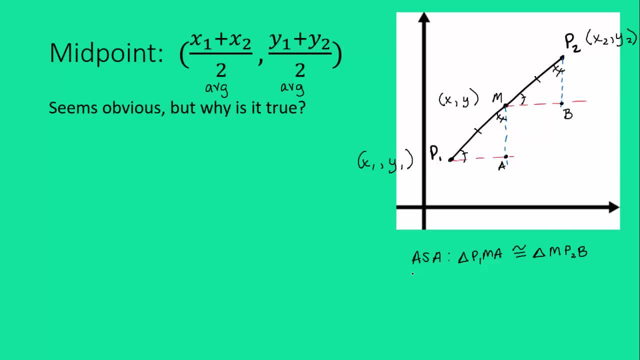 of the triangles, to make some equations using the coordinates and then figure out if we can prove this midpoint formula. So the first thing I'm going to do is look at those two red lines. Not only are they parallel, but now, because they're parts of two, 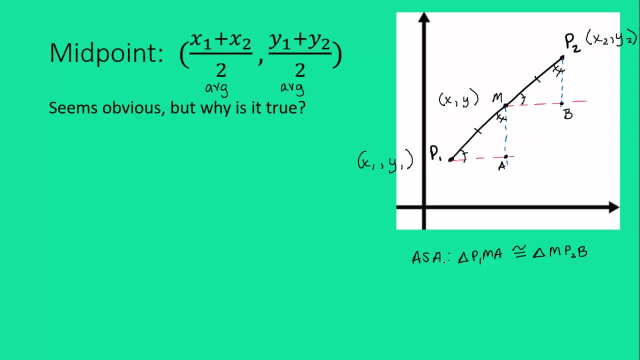 congruent triangles, we know that they are congruent as well. The distance from P1 to A is equal to the distance from M to B. We can also say that those blue line segments are congruent, so the distance from M to A is equal to the distance from P2 to B. 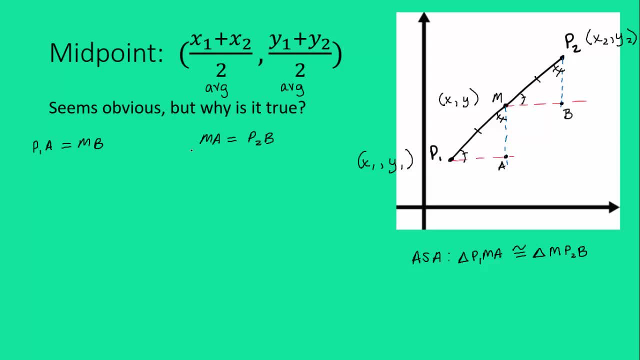 Using those equations. we're going to make equations using our coordinates. We need to name the coordinates for A and B, and we haven't done that yet. So where is A? The x-coordinate for A is lined up with M, So it's x, and the y-coordinate for A is lined up with P1,, so it's y1.. 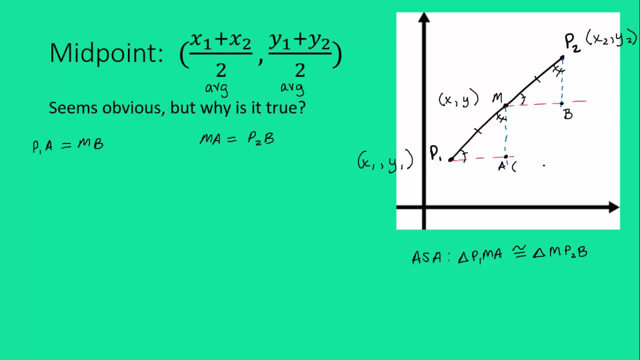 name the coordinates for A and B, and we haven't done that yet. So where is A? The X coordinate for A is lined up with M, so it's X, and the Y coordinate for A is lined up with P1, so it's Y1.. Now B, let's see. the X coordinate is lined up with P2. 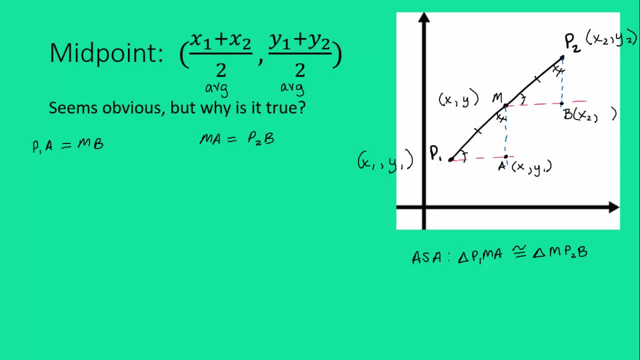 so that would be X2, and the Y coordinate is lined up with M, so it would just be Y. Alright, now I think all our coordinates are labeled and we can start writing some equations here. The distance from P1 to A would be X minus X1, since they're. 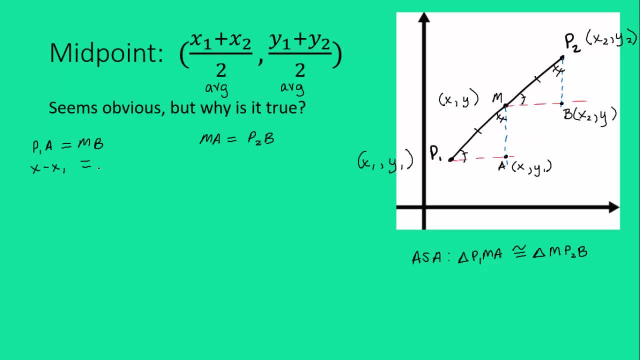 arranged in a horizontal line and the distance from M to B would be X2 minus X. Now let's solve for X. since that's the coordinate of the midpoint, I'm gonna move all my X's to the left and move my X1 over to here. Okay, let's see what we've. 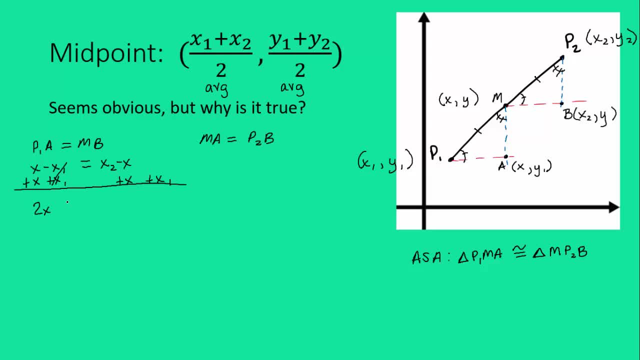 got. We've got 2x is equal to X2 plus X1, and if I divide both of those by 2, you can see that this is pretty much my midpoint formula. Let's clean it up and rearrange it. and there's the X. 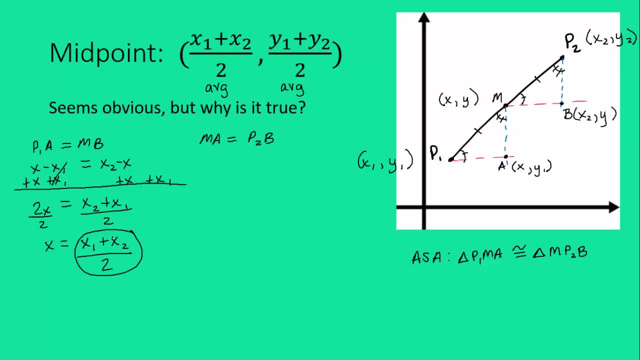 coordinate of the midpoint right there. Let's try the Y's now. The distance from M to A is Y1 minus Y, and the distance from P2 to B is Y minus Y2.. So let's see how could we get our Y's together and our other things away from. 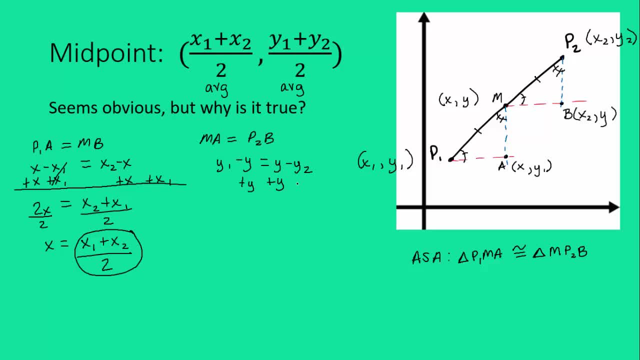 that I'm just gonna move that over there and I'm gonna add a Y2 to both sides and let's see what we've got now. Y2 plus Y1 is equal to 2Y. This looks familiar. right, We can finish it off just like we did with the X's and neat it up a. 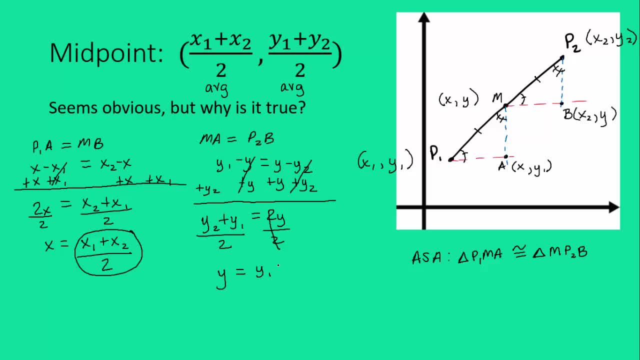 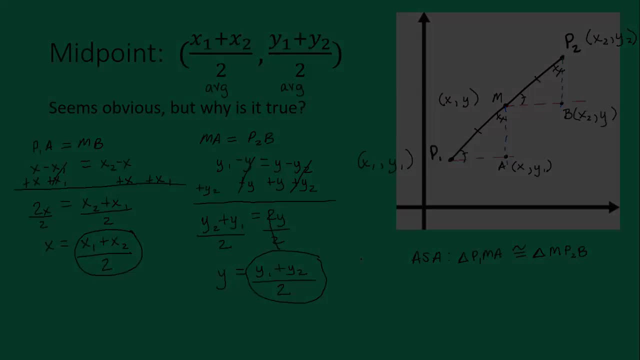 little bit. So Y is equal to Y1 plus Y2 all divided by 2, and there is our Y coordinate of the midpoint and that's our proof of the midpoint formula. Now go use it. 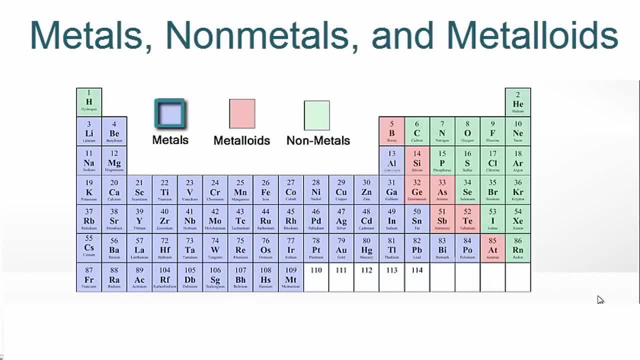 Let's take a look at the metals, nonmetals and metalloids on the periodic table. On the left we have the metals, Then in between them we're going to find the metalloids, And then on the right we'll find the nonmetals. 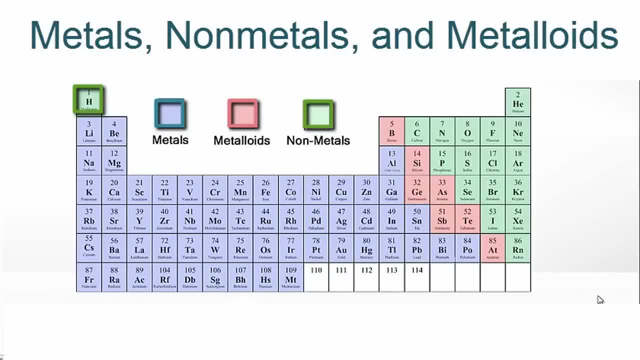 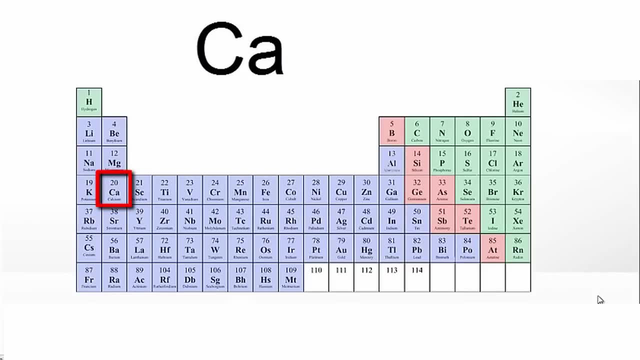 Do watch out for hydrogen, though. It is on the left-hand side with the metals, but it is a nonmetal, So let's try one of these. So calcium, Is calcium, a metal, nonmetal or a metalloid? Well, you can see that calcium is on the left-hand side of the periodic table, so that's going to make it a metal. 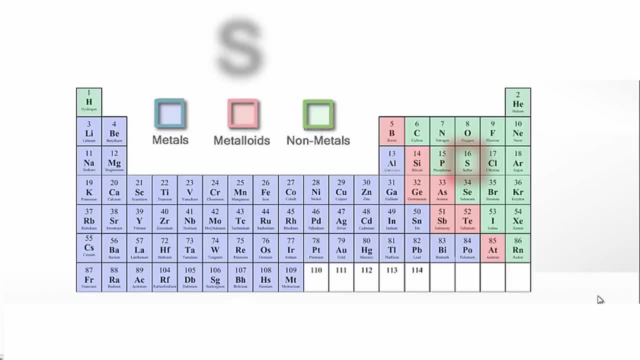 Let's try another one: Sulfur. Since sulfur is on the right-hand side of the periodic table, we know that it's a nonmetal. Let's try one more: Tellurium. You can see that tellurium is in that junction. 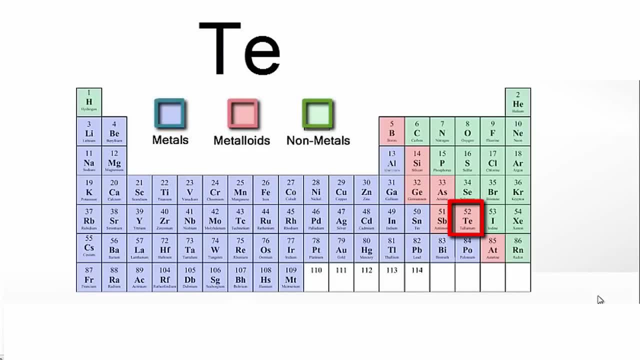 Sulfur is the structure between the metals and the nonmetals, And that's going to make it a metalloid. Finally, let's look at one more: Hydrogen. You might remember that hydrogen is the one that's a little bit tricky.